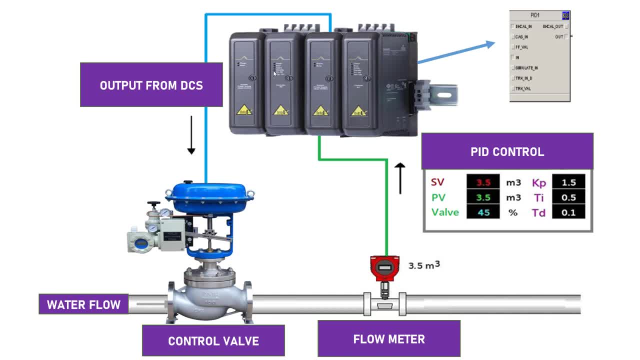 inside that particular controller, Delta VDCS controller. Delta VDCS PID output would be connected to your control wall. Based on the output, you would be deciding how much should be the opening or closing of the wall, based on the requirement of the flow. Before we go ahead, 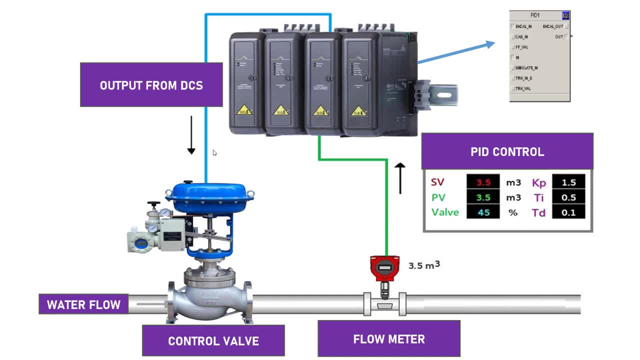 and start working on this particular project. it's important to understand few foundational concepts because once I would be using that, for instance, you see that back calculation input. There are a lot of other concepts like that which are very important to understand for you before we actually talk about the programming side. 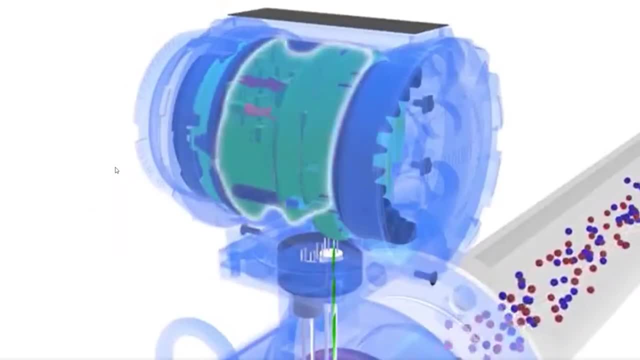 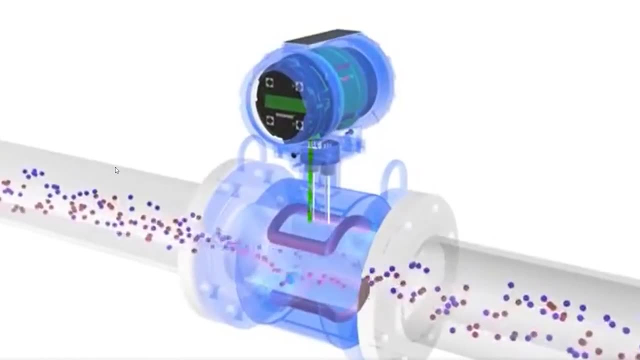 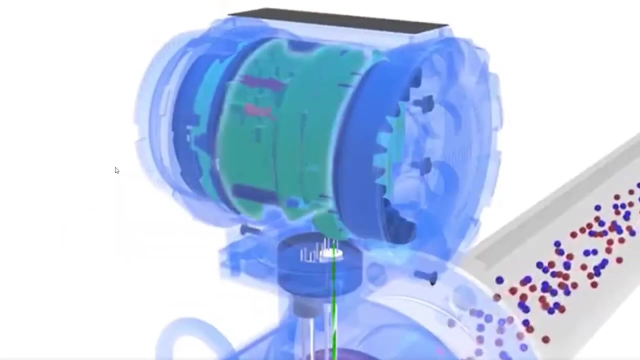 So let's get into the foundation first Concepts I'm going to talk right now are very important. Without that, there is no possibility that you can learn PID in Delta VDCS. You would definitely give up if, in the case, you are going ahead without understanding these concepts Before we talk. 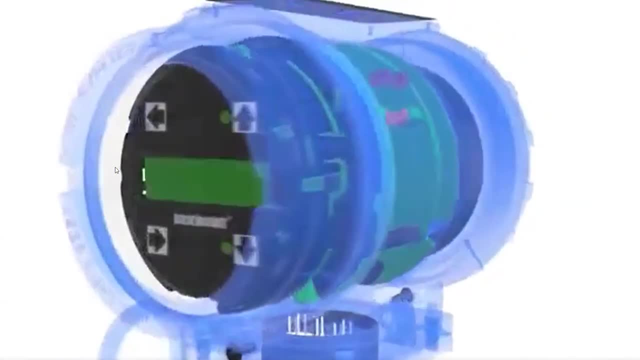 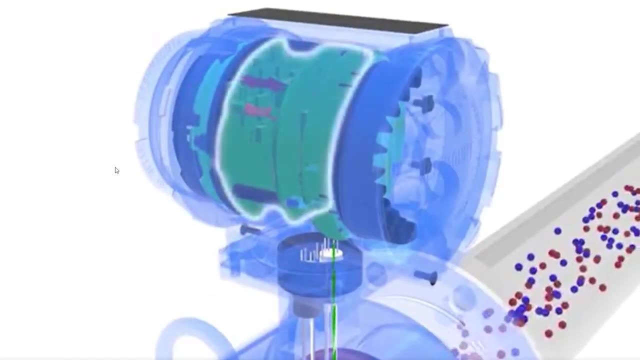 further about it. let's get into the concept of PID. PID is a concept that is very important to understand, So let's talk about today's topic. It's important If, in the case, you like these kind of videos. one thing is very important: One favor you can give us: hit the like button If, in the case, 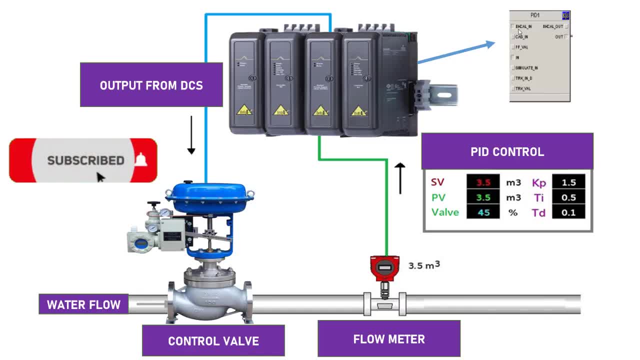 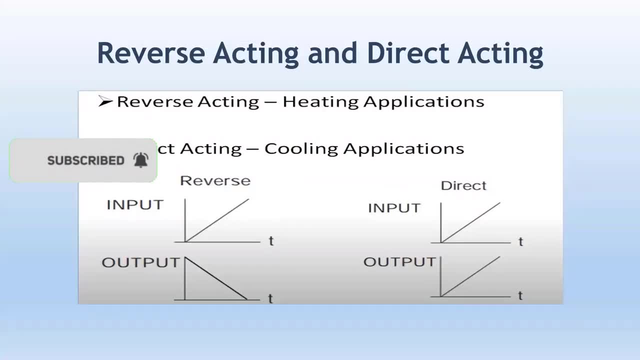 you haven't subscribed to this YouTube channel, consider subscribing. Turn your notification on so that you don't miss any video. Let's talk about the foundation now. So there's two ways: reverse acting and direct acting. What is this when you talk about PID loops, especially in Delta VDCS? 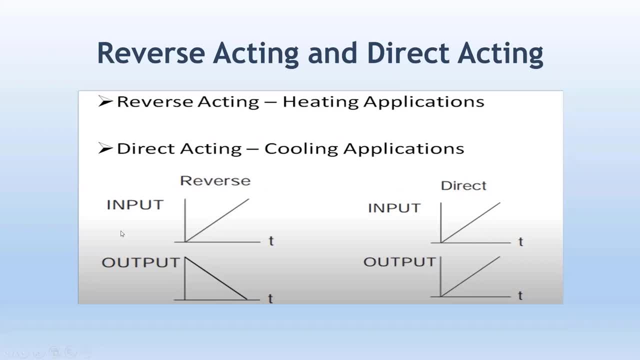 Reverse acting. This guy is there. When you try putting up your input high, this would get down. If you talk about heating application, that's where you have input high, Like if your input, if there is like too much heating already, then what you need to do 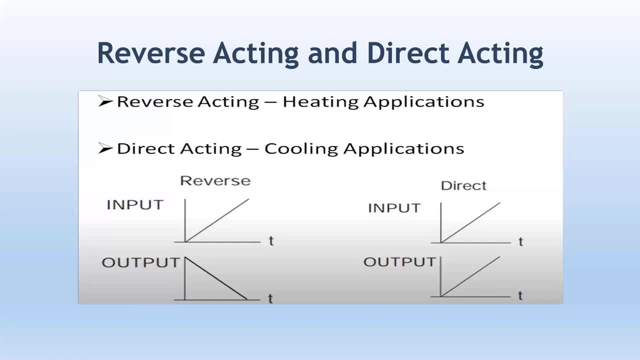 you have to control the heating, Like you have to get your output low right. If there's too much heating, your heater need to be get need to get low right. But when you talk about cooling application, which is when you have too, 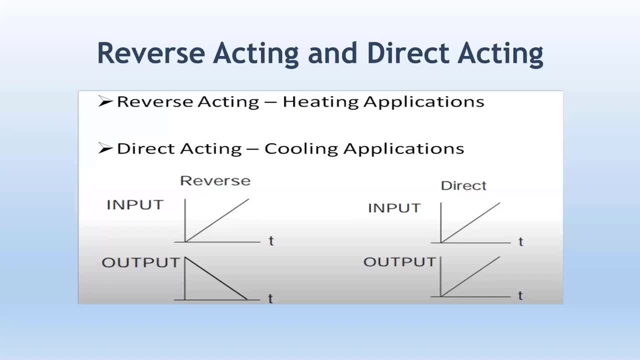 much heat, you should have a too much cooling app you know need to be introduced, Like, for example, there's too much warm, you would put up your AC on more high. So this guy need introduction, that is, in a PLC or PID terms or a DCS controlled terms, especially in PID. this is called 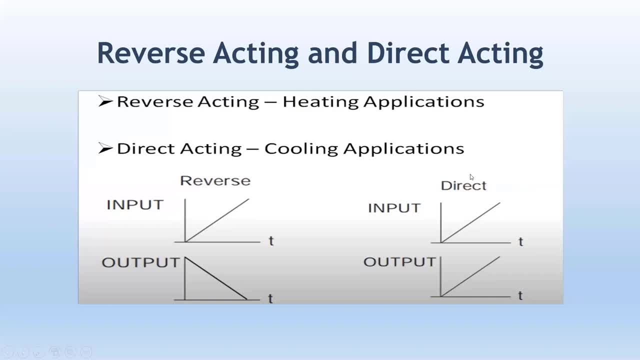 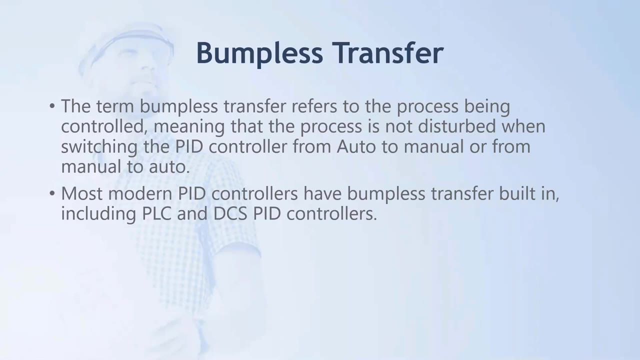 reverse acting And this guy is called direct acting. So reverse acting is when input is getting up, output will get to get low, And then in a direct acting, when input is high, output is high. Okay, So now we have a bump less transfer. What is mean of, what is the meaning of bump less? 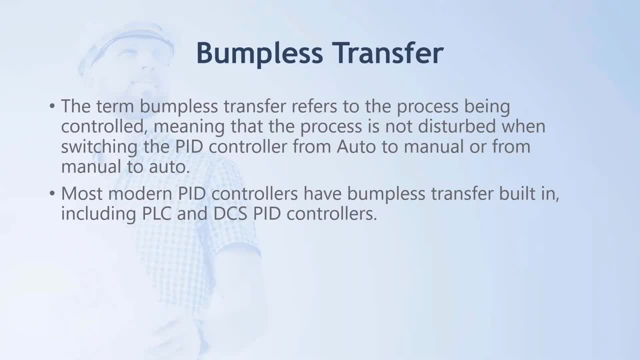 transfer, Because if you don't, if you're not clear about the things that exist in you know, like if you talk about PID tuning, there are a few things that need to be like a PID block, few things that need clear. 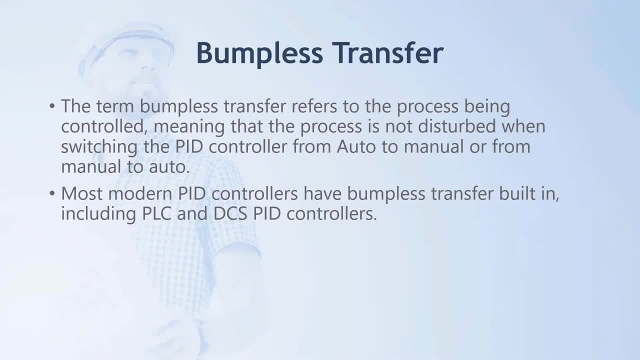 introduction. So I'm just summarizing that information, what is needed. There's nothing on this whole slide set up And you're aware that even in the whole training there was not a single thing which was not in use which I discussed on this training. So this is same here. So when you 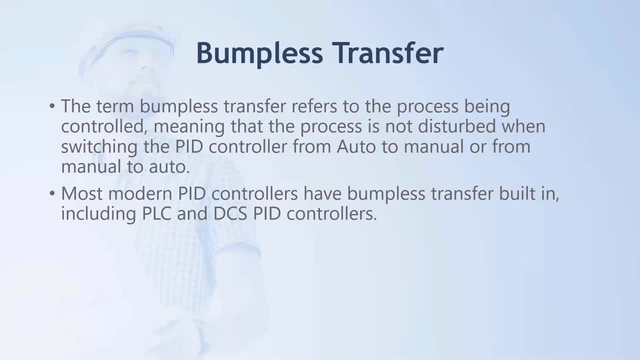 talk about the bump less transfer. the term bump less transfer referred to the process being controlled. That process is not disturbed when switching the PID from auto to manual. Like there is an auto, auto is just by PID and manual is by operator. So when you actually put auto to manual normally 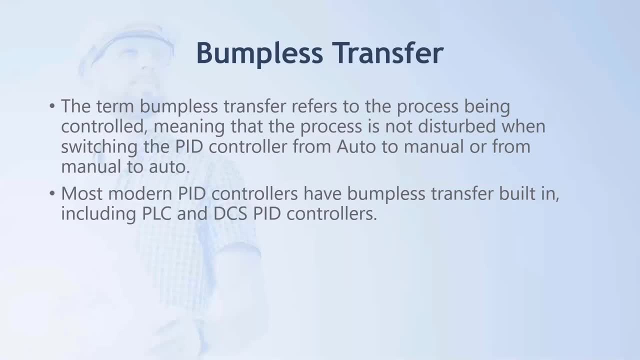 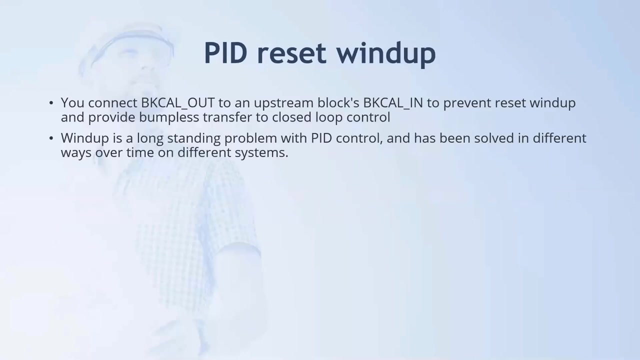 you know your control loop deviate too much. to take care about that, We call it a bump less transfer. That is a process that when you take care about switching of auto to manual or manual to auto and you make it smooth. Okay, the most modern PID controllers have built in bump less transfer. This is very, very important. 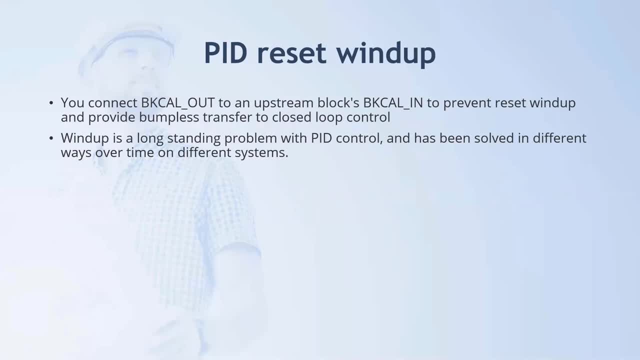 thing. There's a back calculation output and there's a BK calculation in output. there's an output and in. okay, So that need to be connected. back calculation out would be connected to back calculation in. we would see in a PID block when I would be doing it. 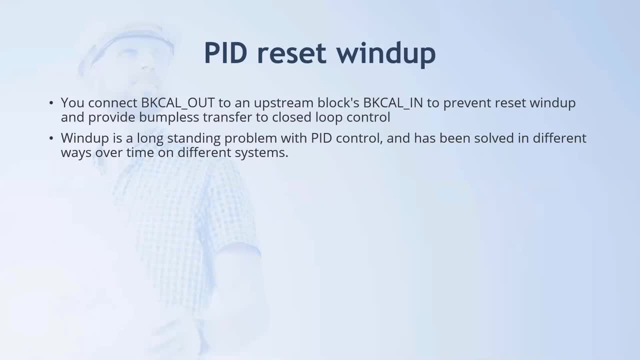 So if you were doing an exercise right in front of you, back calculation out would be connected to back calculation in, and why we need to connect. connected, that's for bump less transfer And then to prevent a reset wind up. Now you would say: what is a reset, wind up? Reset, wind up or wind up is a long staddling problem with. 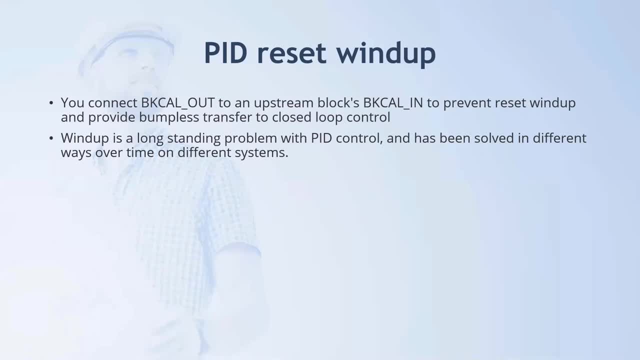 PID control And it has been solved in a different ways over the time on different system. But when you talk about there's a too much deviation between set point and PV and that is pretty longing like your controller is not able to get in your PV close to set point. 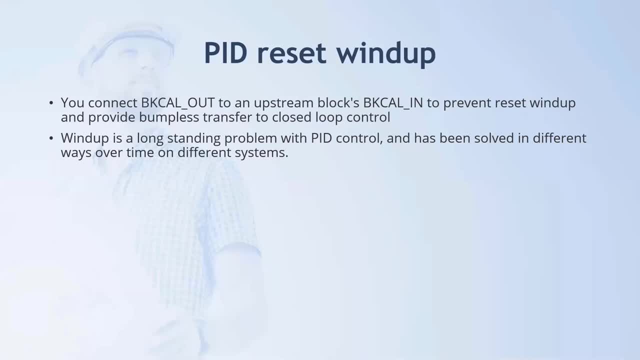 That's what we call it Reset wind up. So that mean like for a long time your problem exists, the error is still there and it's not able to your. your output is getting up but it's not able to actually meet your requirement. That's what we call it reset wind up. 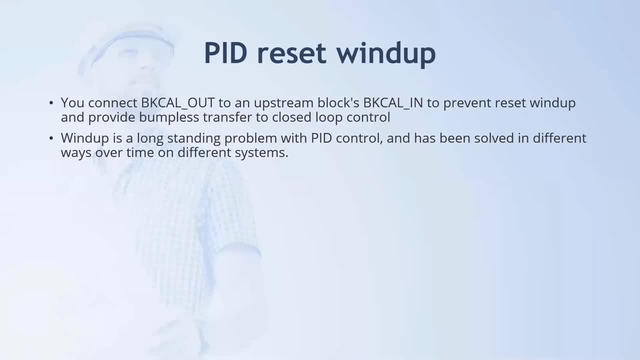 To avoid that, just keep in your mind that back calculation in would be connected to- sorry, back calculation output would be connected to back calculation in. you would see when you would be doing the PID implementation. That's a feedback. In short terms, you can say how much is your output. that would be fed into the block again as an input. 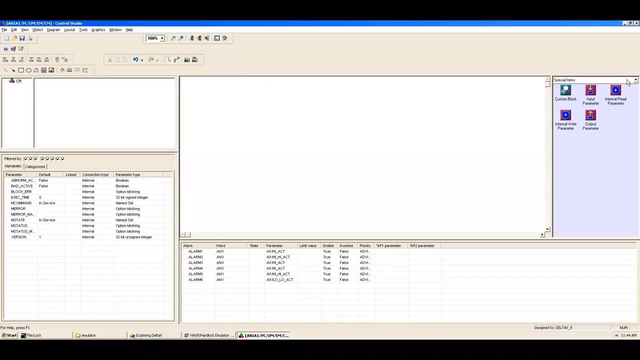 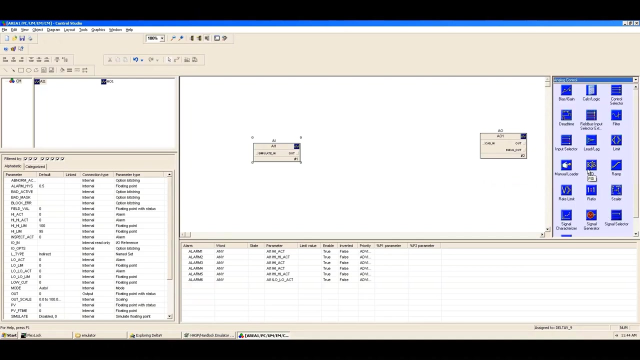 Any questions? Okay, First of all, we need to know, we need to know, we need to know, we need to have in a log input. Okay, and we would put in a log output In advanced control. you would see this PID. 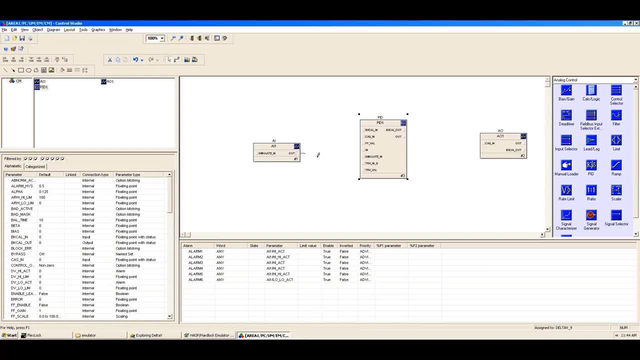 You are going to put it. First thing you would do you would collect, connect that input to output of that simulate in to input of the PID, and then output of this guy would need to be connected here, Gascade, in. Now you see this back calculation out what I was talking about. 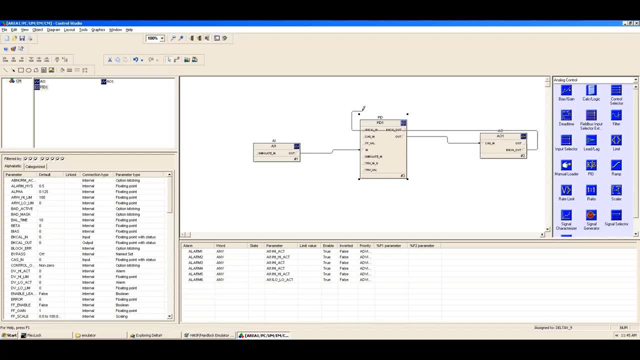 So this back calculation out need to be connected to back calculation in. Okay, So we have a connection from here to this guy. To make it look better, you can do like this: Okay, So this out is connected here and this out is connected to in back calculation in. to white, your reset, wind up and bump less transfer concept. 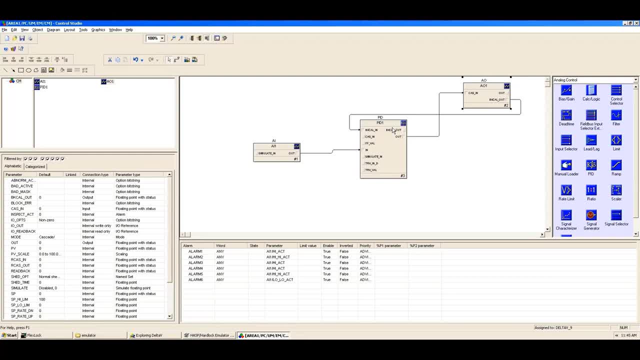 which he actually talked about before. So very important thing now which we really really need to understand, is there are a few things that you have to have here which are not actually there. So how to get up something in a PID which never, which is not existed? 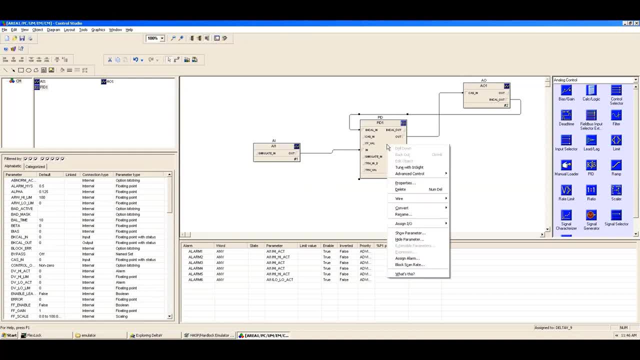 Even you can see. there's no set point here, So you have to click right: show parameter- browse first. First of all you have to understand. I want this parameter to appear at the input side of the PID block, So I selected type as input. 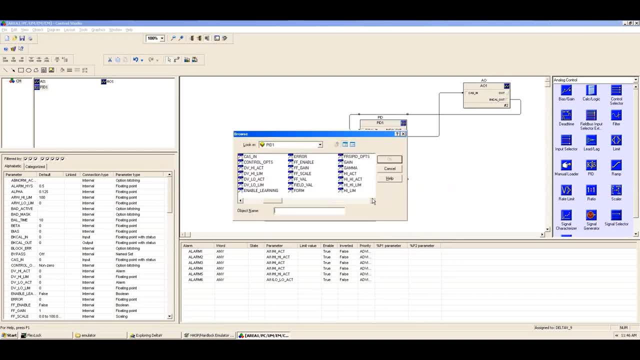 get into the browse Now you have to search for set point. So this set point is right here. Just click OK and click OK. Now you would see the set point is there also right, That's at it. There are a few things that you have to actually take care of when you are going to make a PID loop. 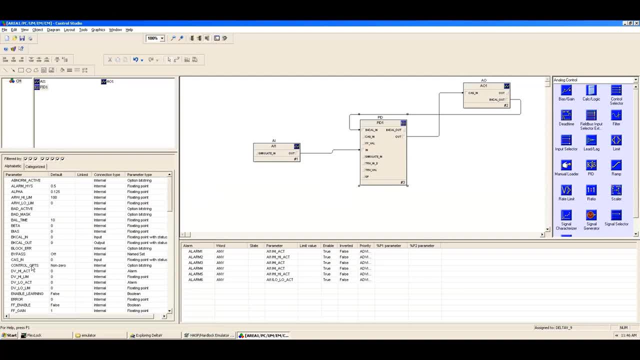 So that is control options. So when you click on this here, you can actually make reverse or direct acting by default. When you haven't selected anything, this is reverse acting, But when you are trying to, you know, select it as a direct acting. 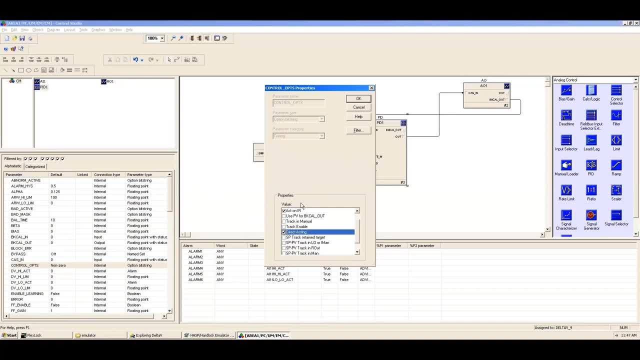 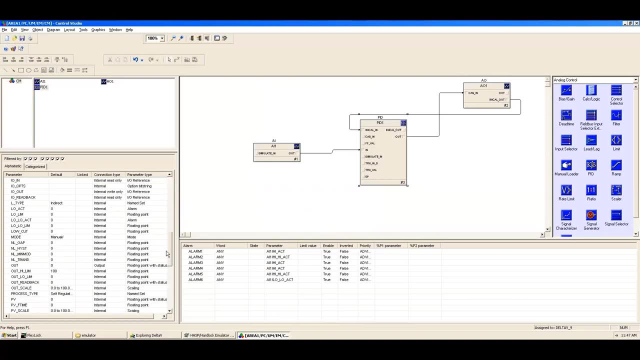 then you can do it like this. You understand the point. So I click on direct acting and click OK. Now this guy is ready. Okay, so good. Now we can give a set point some value. Where is the set point? Set point is here. 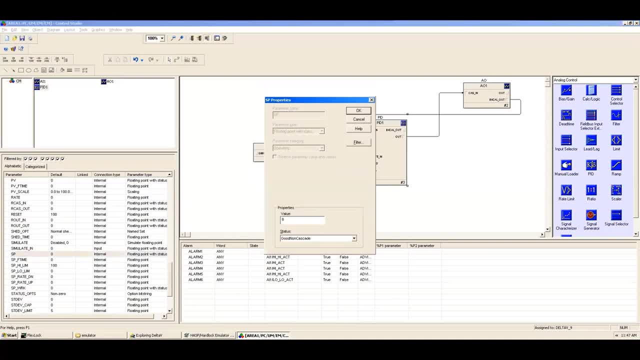 I want my PID to be at 89. And where is the set point? is good, Good cascade, Okay. Then I want this guy to be at some value, right, I don't want this to be set point. I need to give it some value here to simulate in also. 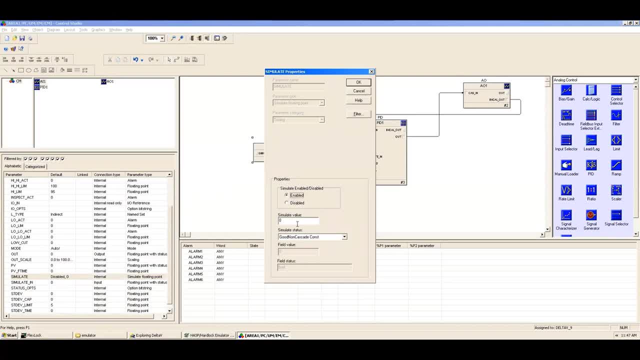 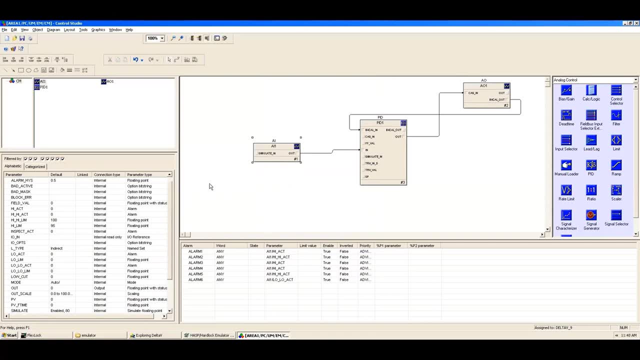 I would enable It. I would give it 80 value. Okay, so this is now 80 value And this set point is termed as your. how much was, how much was the value for the set point 89.. Okay, Now, if we give it a 10 value, 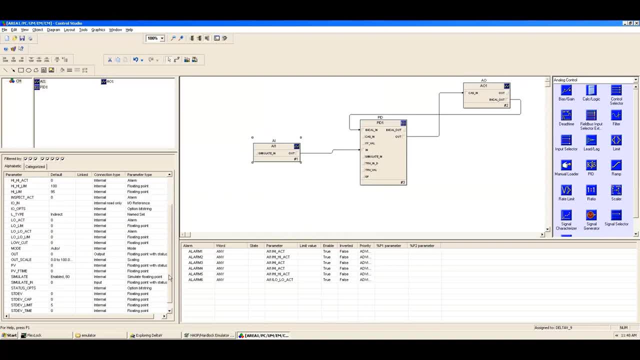 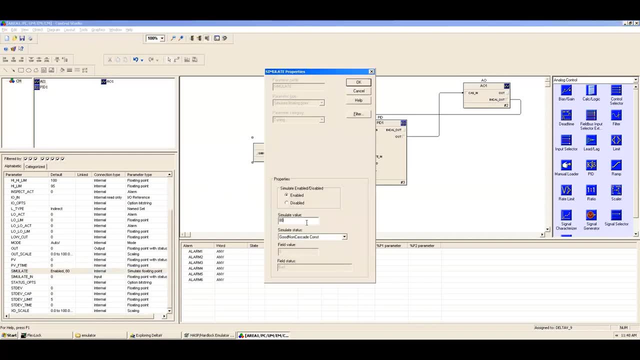 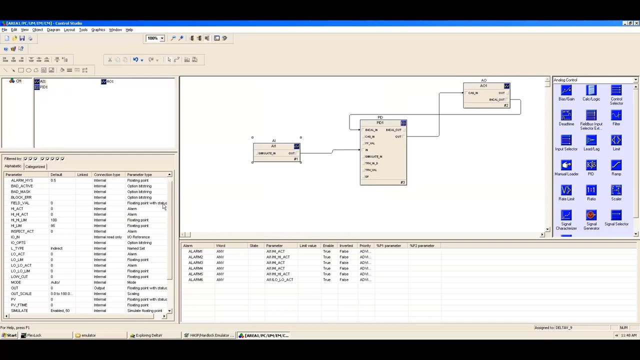 for instance, this AI, that would behave in a better way. I think, Let me, instead of getting a high value, we can give it a Same 6050 when That's a better way. Now you can see there are many options that exist. 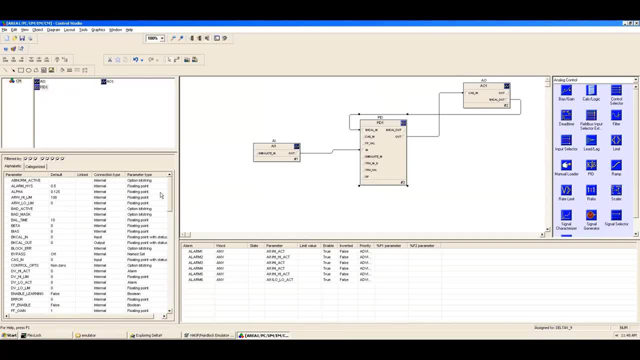 If you come here into this block, you can also see there are many options. But first of all we have to understand. see the gain is there, There is a reset, There is a item P and ID. P, I and D rate is there. 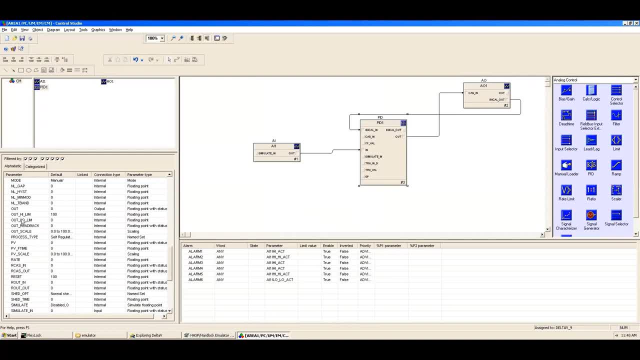 That is there And you have a reset and you have a gain also, And you have a outscale that you have actually scaled a value that your output would be between 0 to 100. It would not exceed more than that. I'm sure that my process value or my control wall is between 0 to 100 percent. 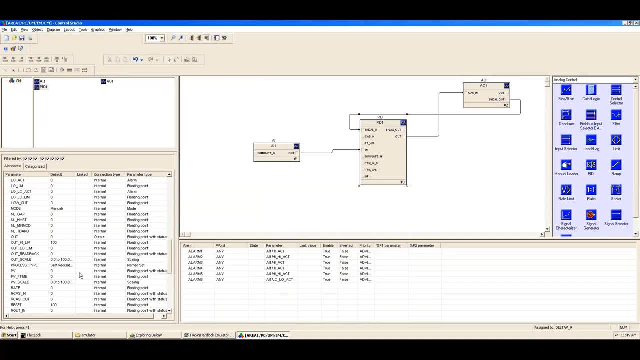 There is no more actually opening of the control wall more than 100 percent, Then in that case, you can see, you can put up a zero limit for a Low limit and high limit would be adjusted to 100.. You can see here. 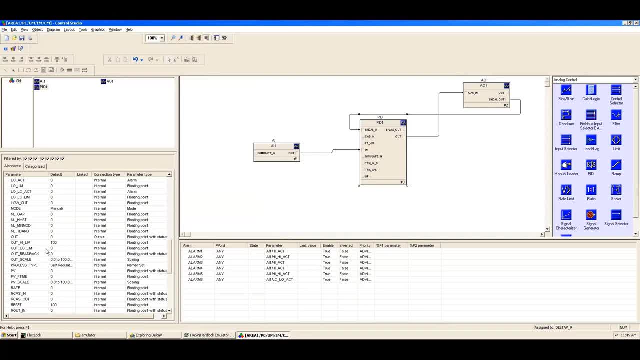 Right, any questions? This, this is your high limit, and similar way, You can also give a low limit and high limit to input values also. But yeah, this is a set point and one important thing with more thing: Yeah, you can see the mode option here. 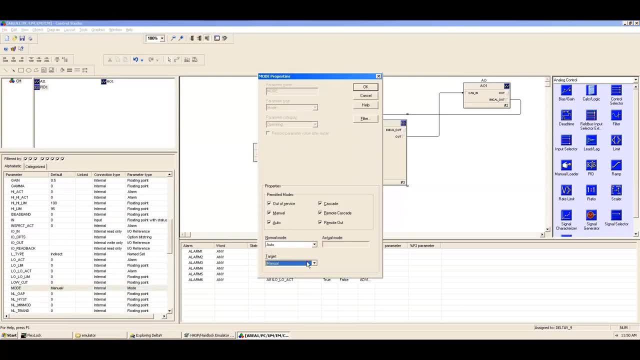 It's in the manual. You can put it Auto, you can put it manual here. You can put it cascade, You can get put cascade remote and remote output. but we would be talking about auto and manual in this case. So I put it in manual and I'm trying to give a value and I need to save this program. 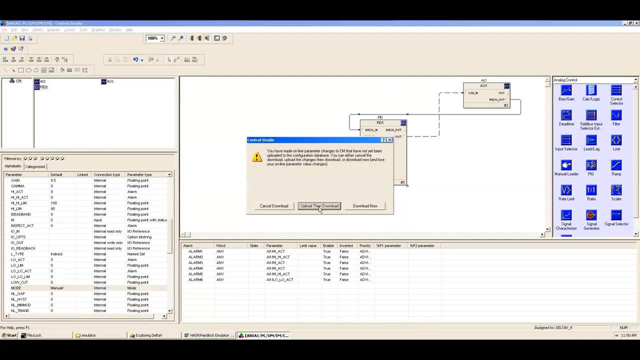 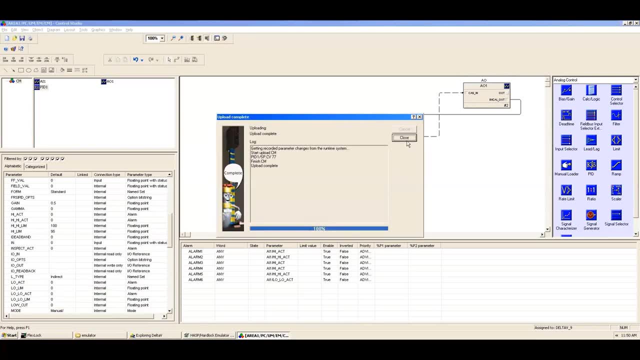 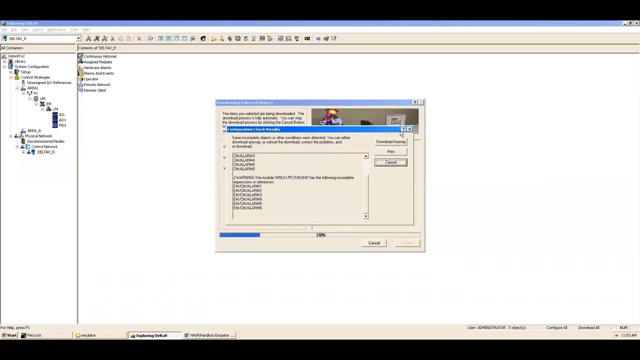 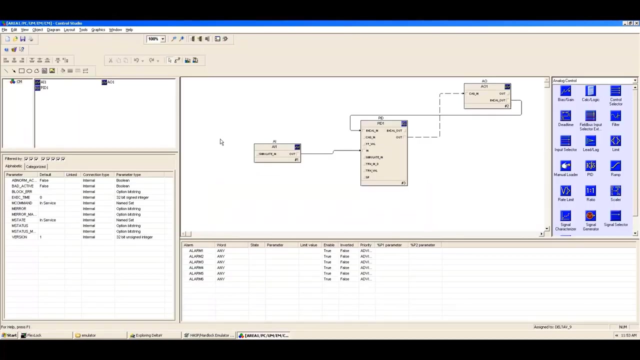 I need to download it And then see what is the response: upload to the download to the station. You can first upload it, select Okay and it's going to upload And then Download anyway, point. So now you see, you put up a value of 50.. 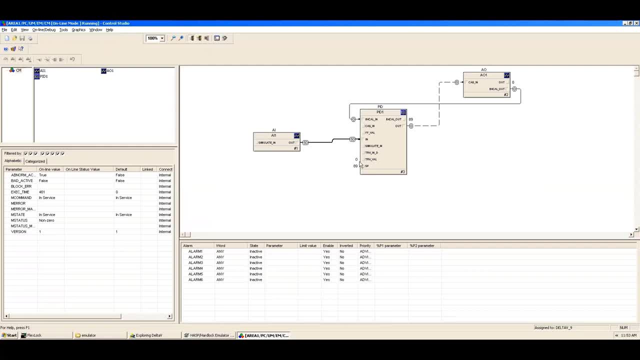 And your set point is 89 as 70.. And you're trying to give the output value to some value. Let's see, and I want to give this output some value, So I'm trying to give out manually, So I'm trying this to be 30.. 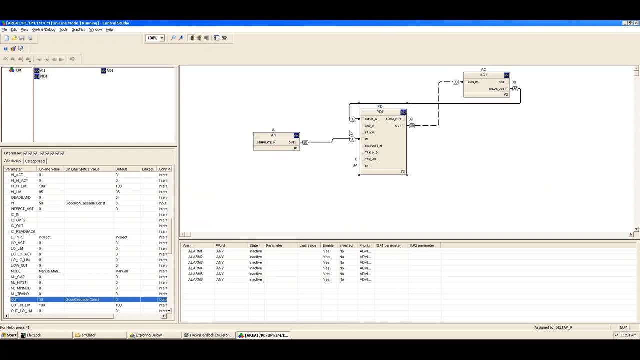 Okay, so I put this output manually: 30 value. Now I'm going to change the mode of operation to automatic to see how it operate. So I select mode and make it into Auto And click. So now we have to tweak with the PID terms to see the response. 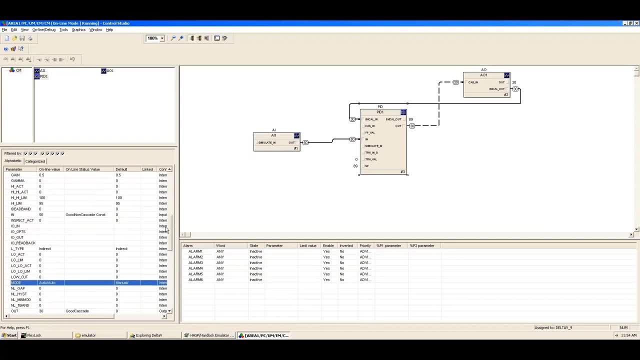 So if you see that we have a gain here, So I want my gain to be high, So what I wear is again the best way is put here and just select Some. give some value and I give it one To see the response now see, the value is changing when I give a cane: gain value. 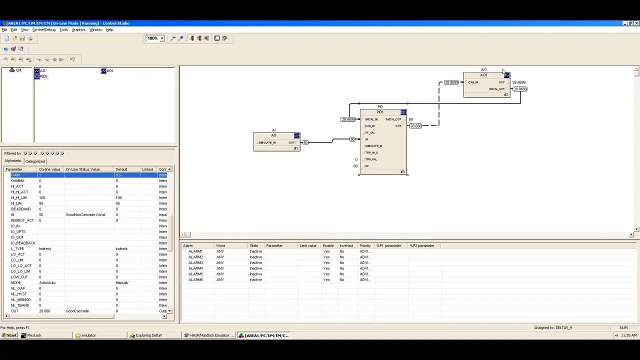 You see, the value of feedback is also Changing and that back calculation is getting back to here Also. you see, that's what I was talking about. The feedback is going to be fed in in the back calculation. No system is trying to reach to that value.